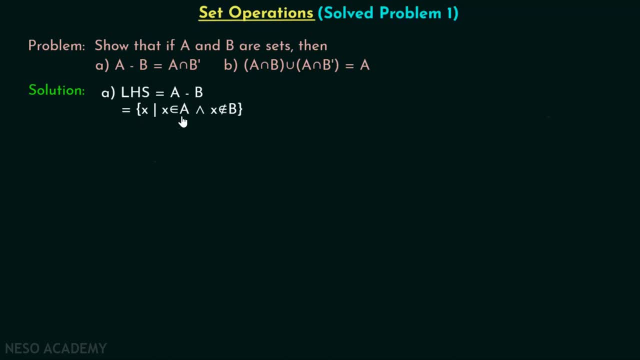 We know that this is nothing but a set of all X, such that X belong to A and X does not belong to B, right Here, obviously, you can rewrite this X does not belong to B as not of X belong to B. X does not belong to B means not X belong to B, right. 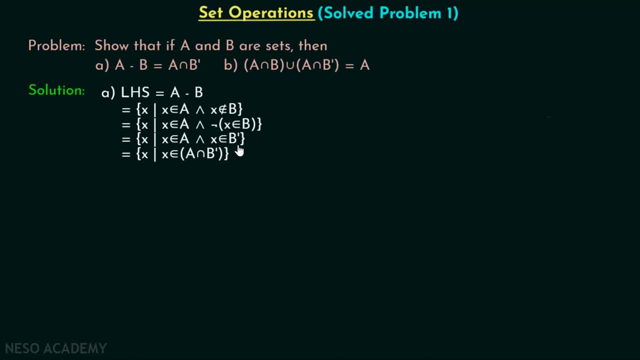 We can rewrite this as X belong to B complement. Obviously, X does not belong to B means X belong to B complement. So this is the resultant set, That is, a set of all X, such that X belong to A and X belong to B complement. 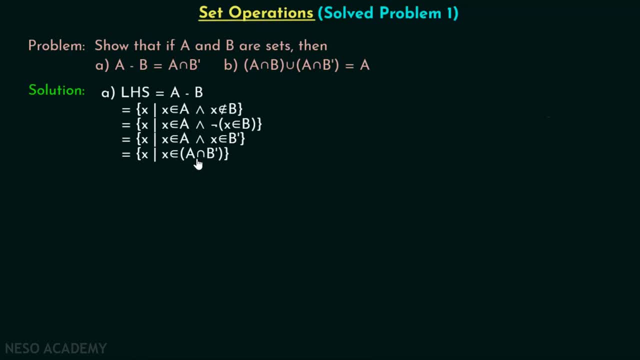 We can rewrite this whole sentence as X belong to A intersection B complement. Isn't that so? Because here we have an AND operator. This is X belong to A and X belong to B complement. We can say that X belong to A intersection B complement, right. 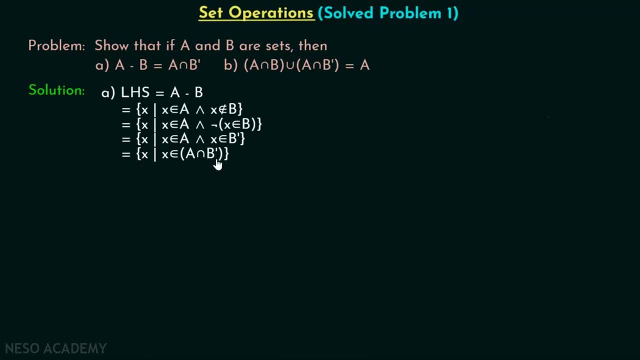 So we have a set of all X such that X belong to A intersection B complement, which means we are talking about the set that is A intersection B complement And obviously this is RHS right. So we have deduced RHS from LHS. 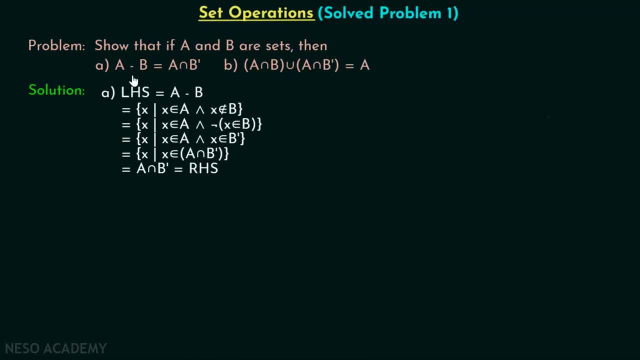 Thus we can say that LHS is equal to RHS and hence A minus B is equal to A intersection B complement. right Now let's just try to prove this: That is A intersection B union, A intersection B complement, equal to A. 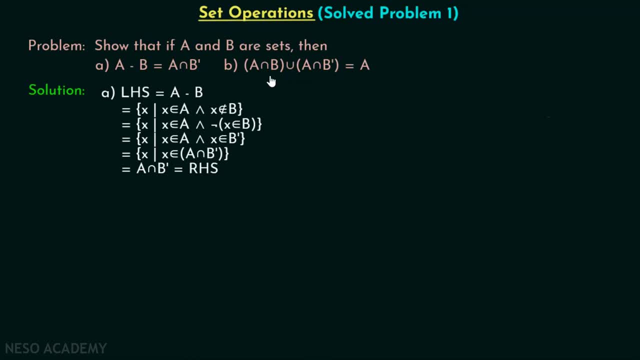 For this. we will take the LHS part and we will try to deduce the RHS from LHS. Let's take the LHS part first. That is A intersection B union, A intersection B- complement. Now this is nothing but a set of all X, such that X belong to A intersection B. 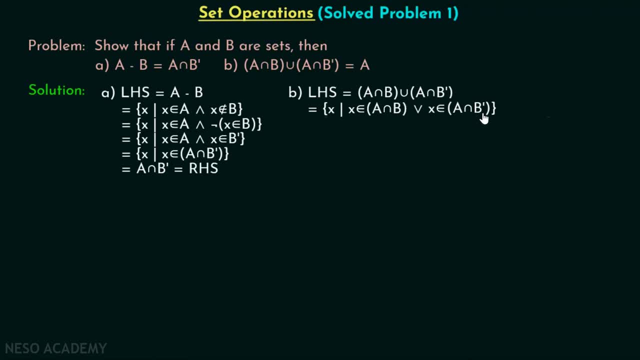 or because of union, X belong to A intersection, B complement right. Obviously, X belong to A intersection B can be rewritten as X belong to A and X belong to B. X belong to A intersection B complement can be rewritten as X belong to A and X belong to B complement. 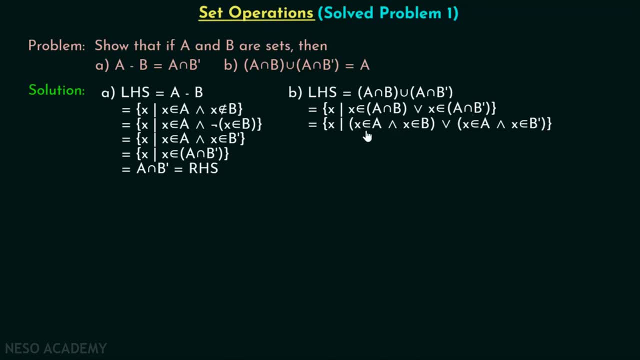 Here we are talking about intersection, right? So and must come in between these two, and obviously these two as well. From the distributive law of logical equivalence we can say that P and Q or R is nothing but P and Q or P and R. 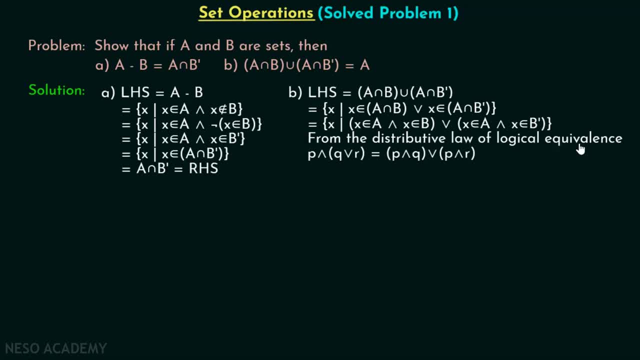 This is true right. This is from the distributive law of logical equivalence. You can see here that this is: X belong to A and X belong to B, and here we have an OR operator. then we have X belong to A and X belong to B, complement right.